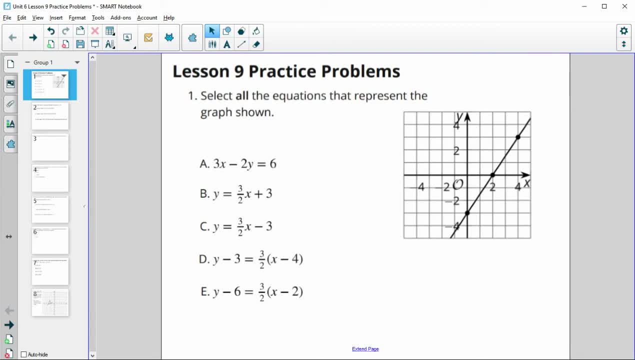 In this video we're going to take a look at the Unit 6, Lesson 9, practice problems. So number one says: select all equations that represent the graph shown. So when we're writing equations of lines, remember that we'll be needing the slope And remember the slope is going to be. 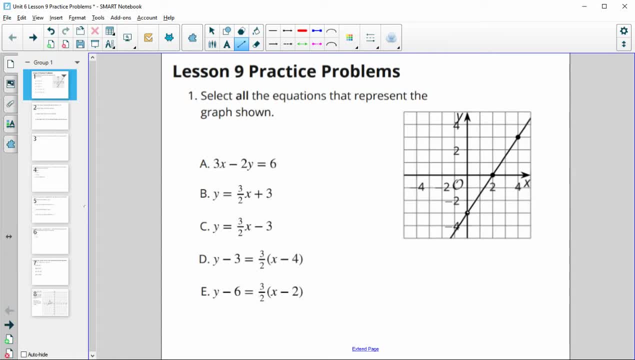 the rise over the run from consecutive points. So let's see- let me make this a little bit thicker here. So we would want to count the vertical distance versus the horizontal distance and simplify if necessary. So for this one, our vertical distance is three and our horizontal. 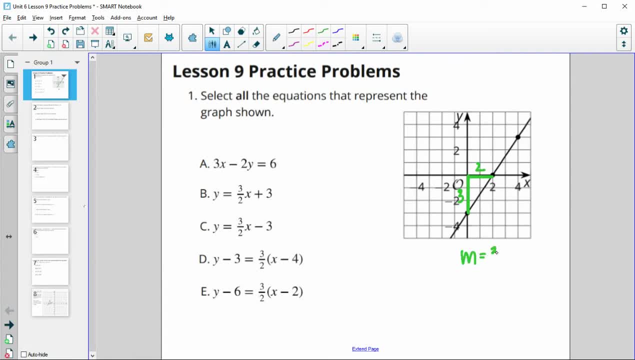 distance is two, So our slope is going to be three halves. And then there's a couple different ways that you can write equations of lines. One that you looked at specifically in Lesson 9 was point-slope form, And in point-slope form you do: y minus the y-coordinate equals the slope times x minus the. 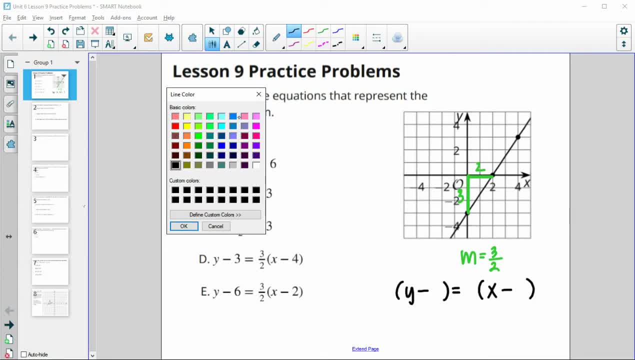 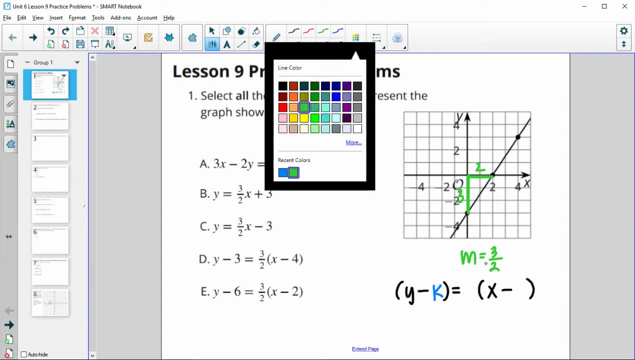 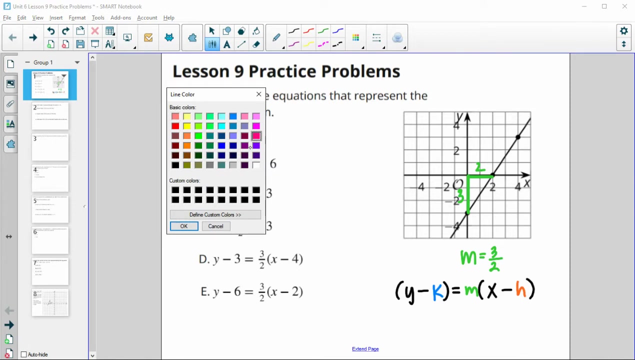 x-coordinate And that's the y-coordinate of any point that you know. So we call it k, And then the slope of the line, And then x minus any the x-coordinate that you know, which we called h. So if you look at this picture here, we see a couple of points that they highlight. 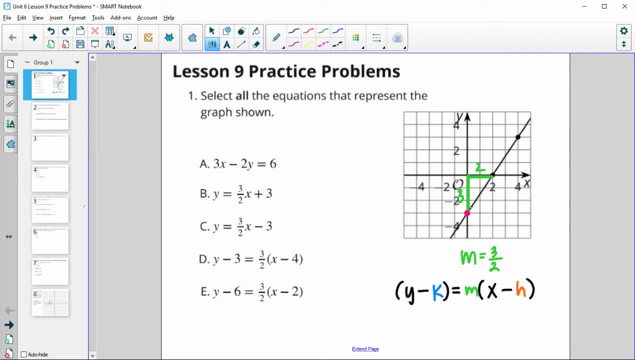 for us that we know. So we know this point at 0, negative 4.. We know this point at 2, 0.. And we know this point at 4, 3.. So you could kind of plug any of these into point-slope form. 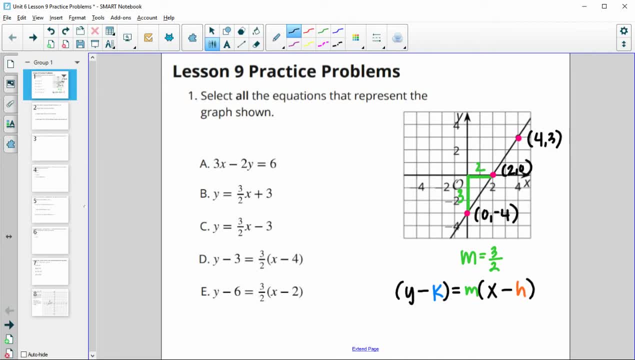 using those points and the slope of three halves. So let's take a look at the options that they give us over here and see if any of them match. So if we look at D and E, these are both in point-slope form, And so the x-coordinate in this one is 4.. The y-coordinate in this one is 3.. 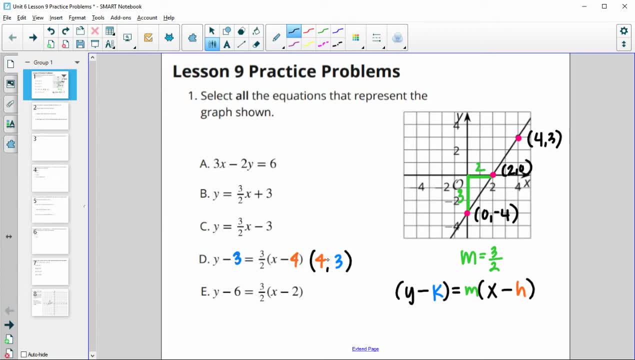 So this is telling us that this line is going through the point 4, 3.. And then we also see that they give us a slope of three halves, So that all matches Okay. so D is definitely an equation of this line. So let's take a look at E. 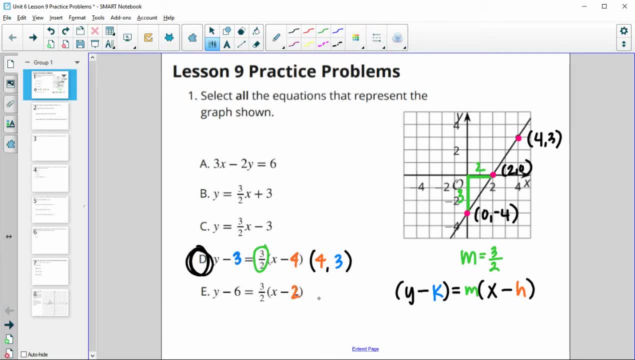 So E gives us an x-coordinate of 2.. And it gives us a y-coordinate of 6.. So we would check and see if that point is on our line. So the point 2, 6 is definitely not on our line. So this one is not an equation for this line. 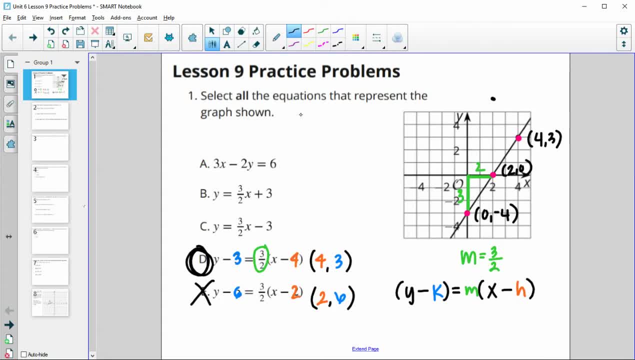 Then other equations that you've looked at in the past are slope intercept form. So that's y equals mx plus b, And so m being your slope and then b being your y-intercept where the line crosses the y-axis. So if we take a look at this one, we already know 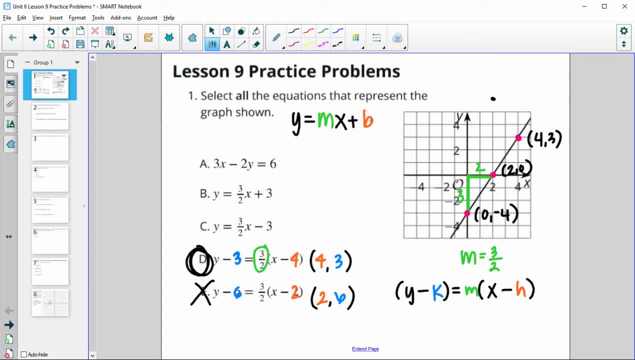 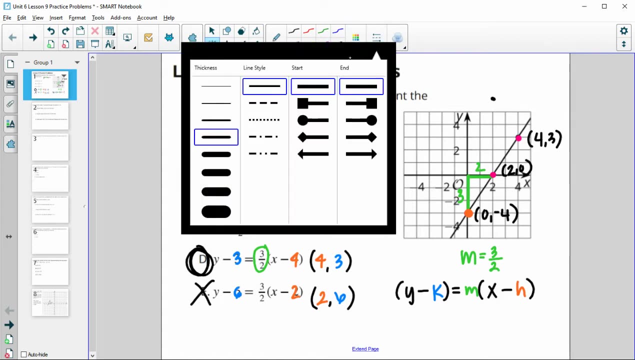 the slope should be three halves, Okay, and then this b would be where the line crosses the y-axis, So this specific point where it actually crosses The y-axis. So that's right here, And so that b value is negative, 4 in this case. 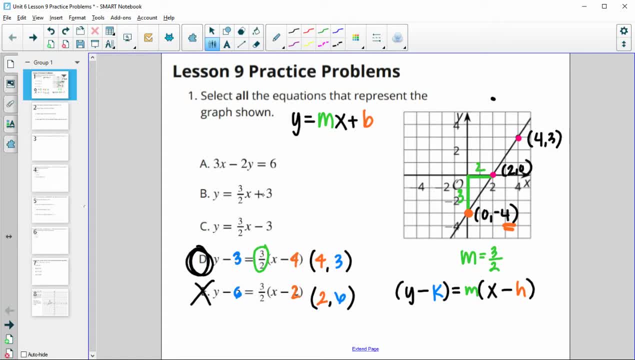 So we can take a look at three halves slope. It needs to cross. Oh sorry, negative 3.. I have this labeled wrong. This is the point 0, negative 3.. So should be crossed. The b value should be at. 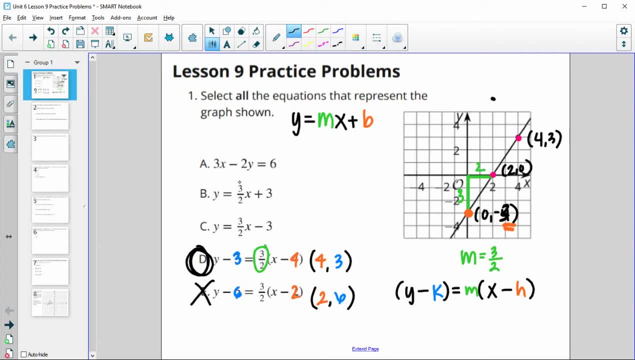 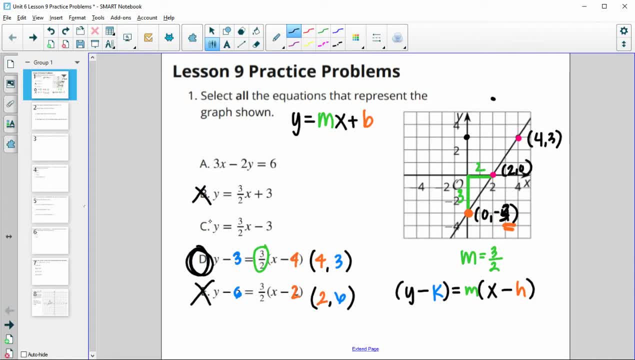 This one has a slope of three halves with a y-intercept of negative 3.. That one is good. So then we have this last one here that we want to work with. So you have a couple options. You could plug in two points, Okay, and make sure that two of these points work on this line. 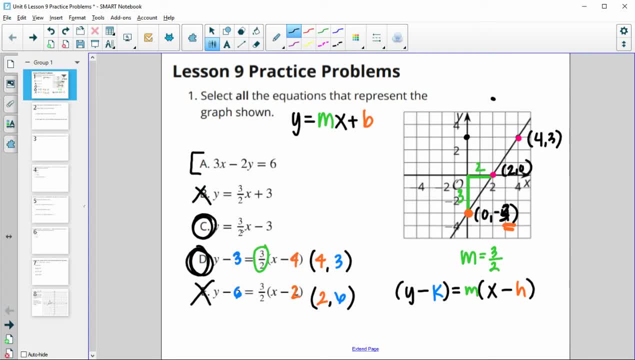 We could also take this slope intercept form that we know and we could manipulate it. So we've got y equals three halves x minus three, And we don't see any fractions in this. So we want to get rid of this denominator of a two. So we could multiply this equation, everything by two. So multiply the. 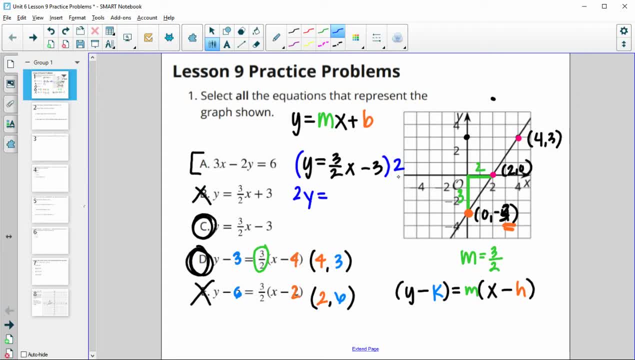 two to the y, and we'd get two y Multiply two times three halves. So let me just do that over here. So three halves times two, that's six over two, which is just three. So two times three halves is three x, and then two times negative three is negative six. So then we could subtract the. 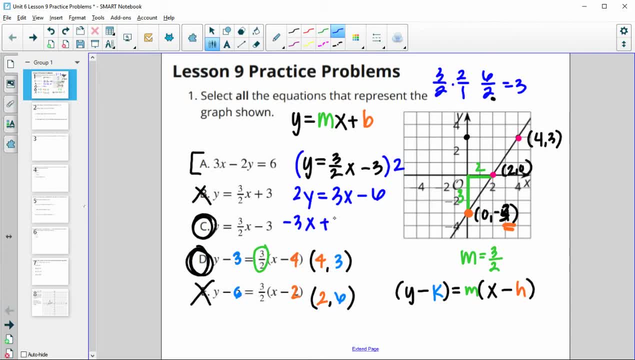 three x to the other side. So we have three x plus two y equals negative six, And we see that this one looks really close to it, but the numbers are all opposite. So we could just divide everything by negative one And that would get us to positive 3x. 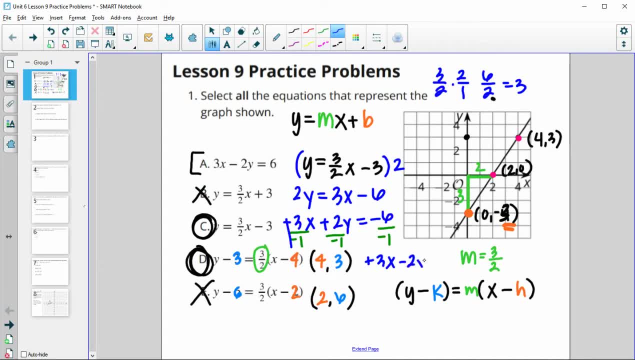 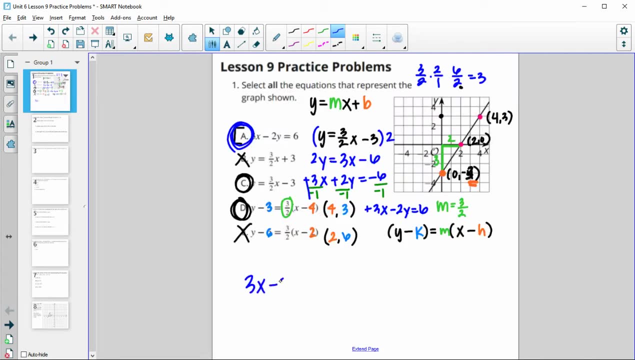 minus 2y equals positive six. So this is in fact a good equation. Another thing you can do in standard form, which is what this one is. So 3x minus 2y equals six. You can look at the x and y intercepts. 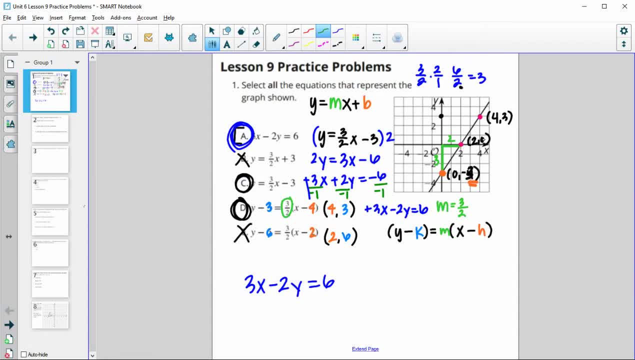 And that's where it crosses the x-axis and the y-axis. So the x-intercept to zero. we know that the y-coordinate is zero. So if we plug zero in here, okay, we would get 3x equals six. divide by three and you get x equals two. 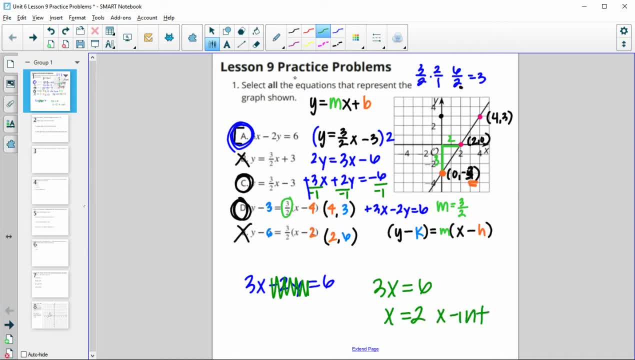 So your x-intercept is two. Then we could do the same idea for the y-intercept. So at the y-intercept we know that x is zero, So we could plug zero in for x, which means that that's zero. 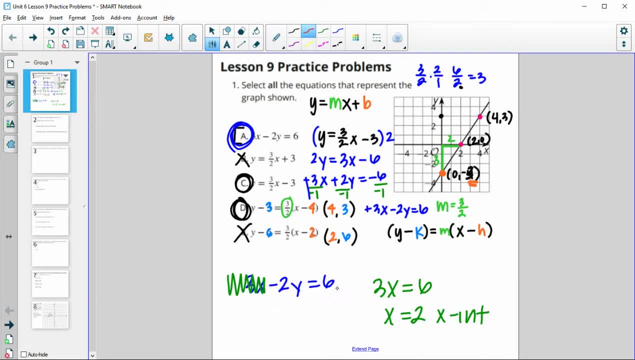 So we just get negative two equals six. negative 2y equals six, So we could divide by negative two And then we get y equals negative three as our y-intercept, And so we could see that the y-intercept is negative three. 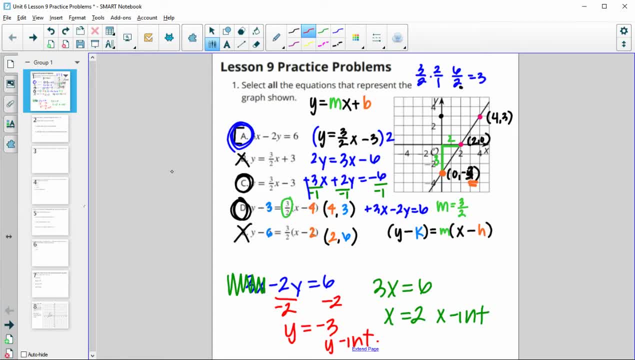 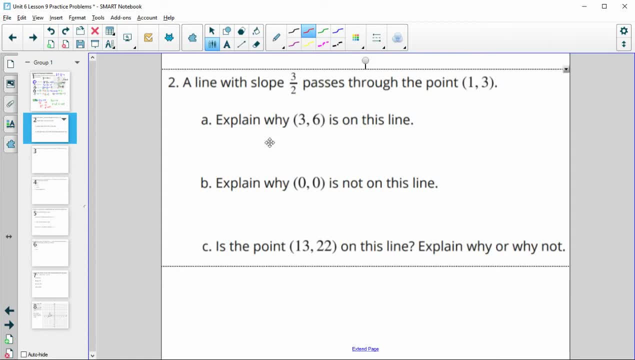 and the x-intercept is two. So that's another way that that's a good problem, All right. number two: a line with a slope of three halves passes through this point. Explain why three six is on the line. So remember that if the slope is three halves. 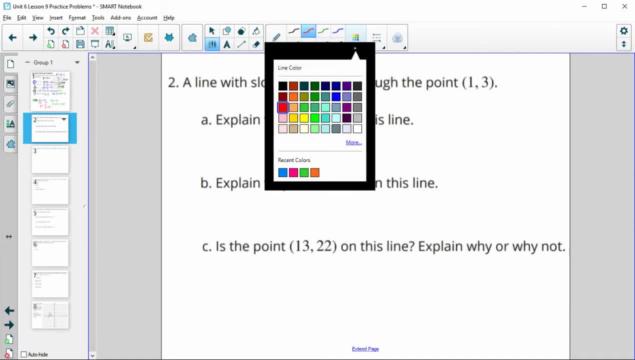 then the slope between these two points should be three halves as well. So remember, slope is the vertical distance. Okay, so when we subtract the x, we're going to get x plus three, the y's, so six minus three over the horizontal distance, which is when we subtract the x's. 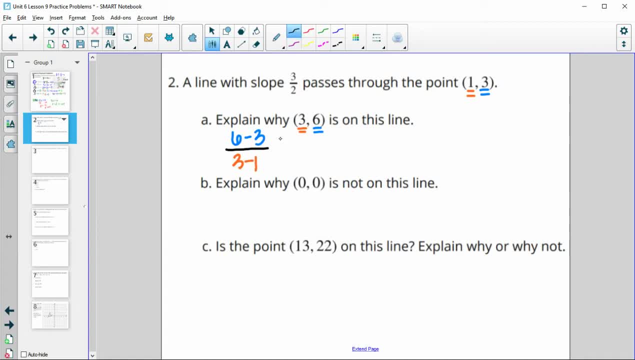 so three minus one, that should equal our slope. okay, so let's see what it does equal. so six minus three is three. three minus one is two. three halves is equal to the slope that they gave us. okay, so this one is on the line um, because the slope between the points 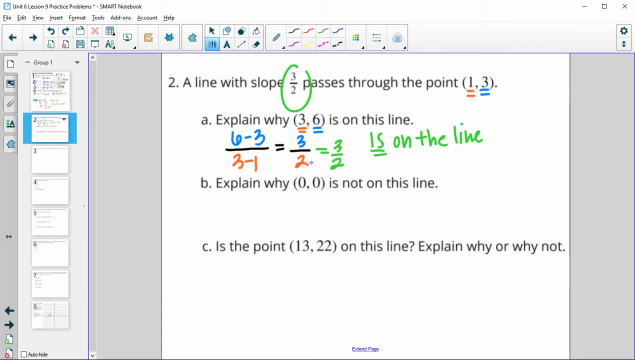 the point on the line and the given point is the same as the slope. so then, why would zero, zero not be on the line? okay, so we can do a similar idea. so subtract the y's so zero minus three, so the slope between this point and the one that's on our line. 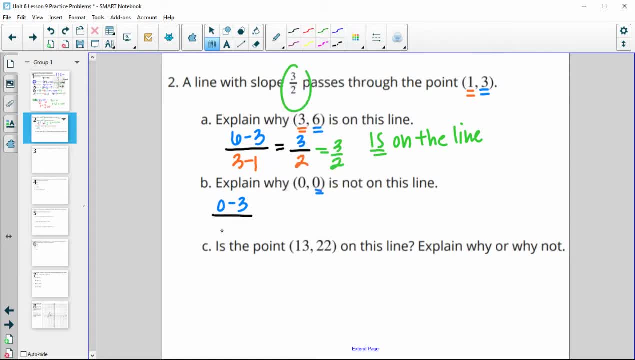 should be three halves, like they told us. so then we'll subtract the x's zero minus one and we get a slope here of negative three over negative one, which is three and three does not equal three halves. so this one is not on the line because the slope isn't three halves. 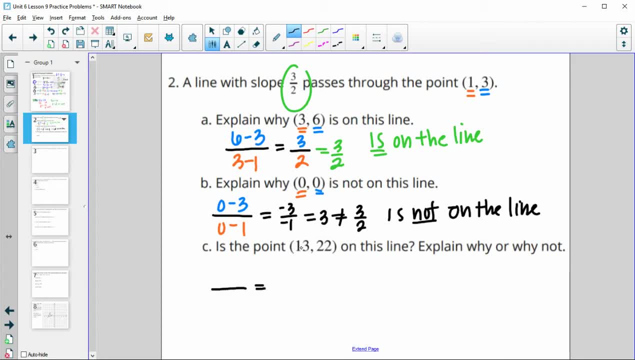 then let's decide. if this next point is on the line, okay, so is the point 13, 22 on the line. so let's look at the slope between this point and the point that we know is on the line. so 20, two, two can be a. one to look at the vertical distance, 13 minus one. to look at the horizontal distance, 22-3 is 19.. 13-1 is 12. that does not equal three halves, so this one is not on the line. number three: write an equation of 5 against 5, 2, 1, 3. that doesn't equal three halves, so this one is not on the line. 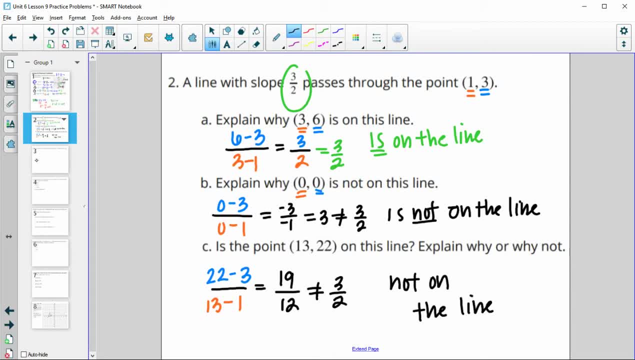 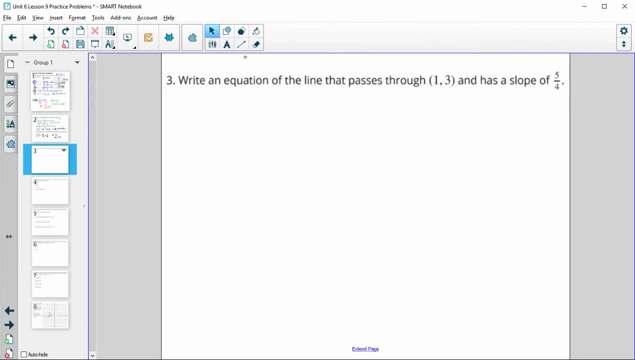 remember. you know this question is qualsi's question. it's my toch quarter to have you, so let's go off of it. try to make one too. Rewrite an equation of a line that passes through this point with this slope, So let's use point-slope form. 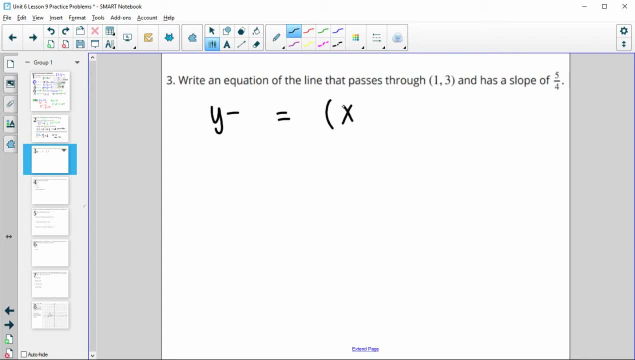 So it's y minus the y-coordinate, equals the slope times x minus the x-coordinate. So the y-coordinate of the point that we know is 3, so y minus 3.. The slope that they give us is 5 fourths Times x minus the x-coordinate of the point, and you have your equation. 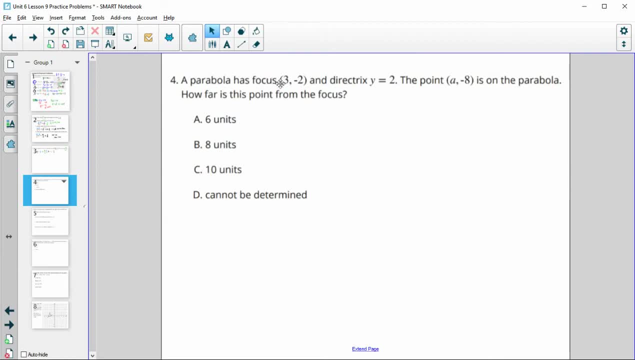 Number four: we have a parabola that has a focus at 3, negative 2 and a directrix of y equals 2.. Then there's a point: a negative 8 is on the parabola. How far is the point from the focus? 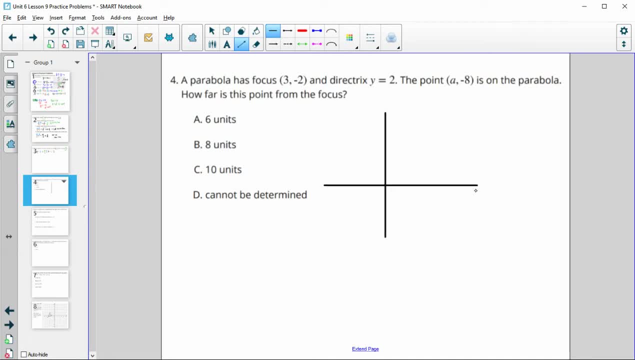 So remember, when we're talking about parabolas, okay, the focus- so let me plot this focus- is at 3, negative 2.. Whoops, Okay. so here's our focus: at 3, negative 2.. And then our directrix is at y equals 2.. 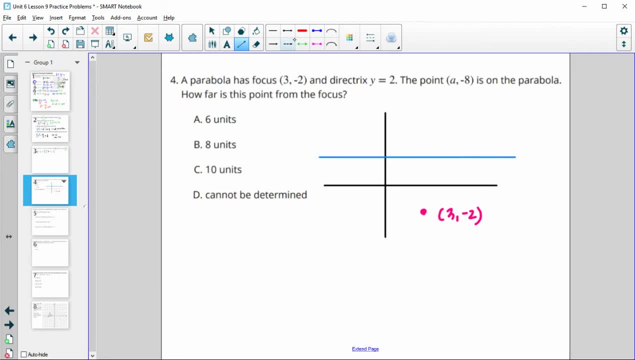 Now remember the distance from this point to the directrix. okay, so the distance from this point to the directrix is the same as the distance from the point to the focus. Okay, so we don't know the x-coordinate of this point. 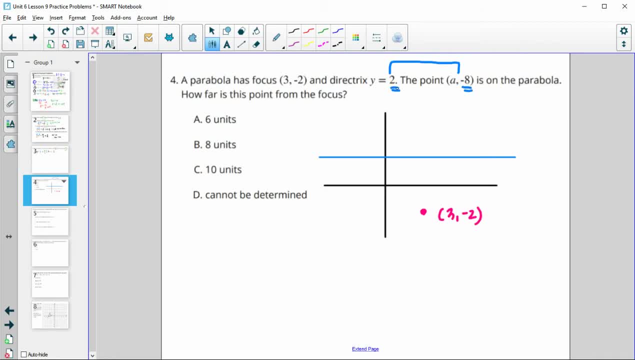 but we do know that it's at a y-value of negative 8.. So if this point- let's say it was here, okay at. let's say this is where a negative 8 was the distance to the directrix. 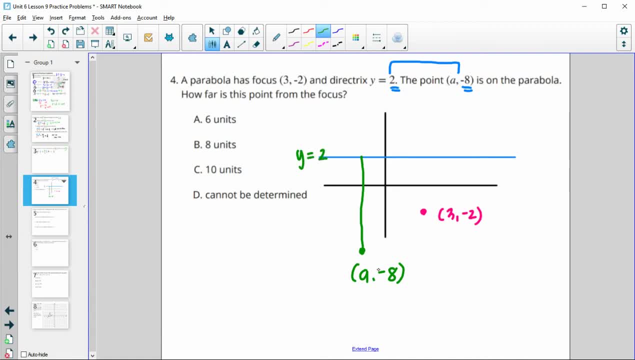 okay, so this directrix line is: y equals 2, how far is negative 8 from 2?? So the distance from negative 8 to 2, you can do 2 minus a negative 8, and you get 10.. 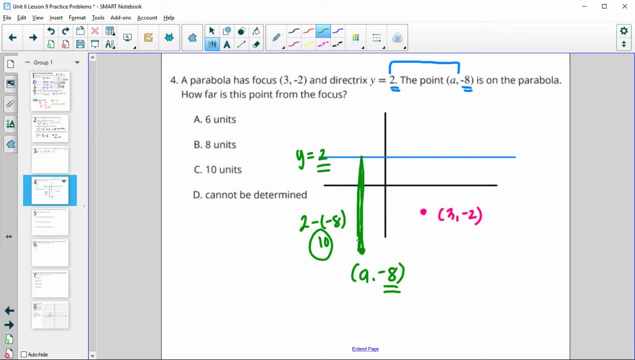 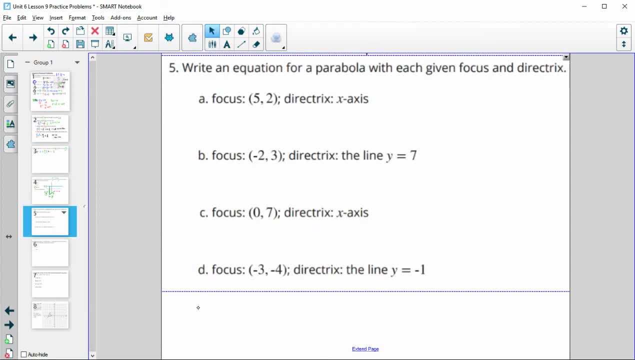 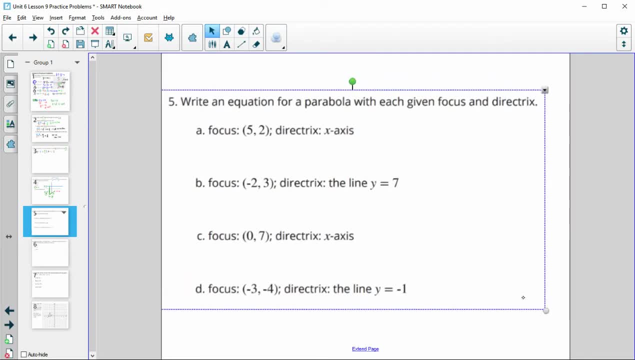 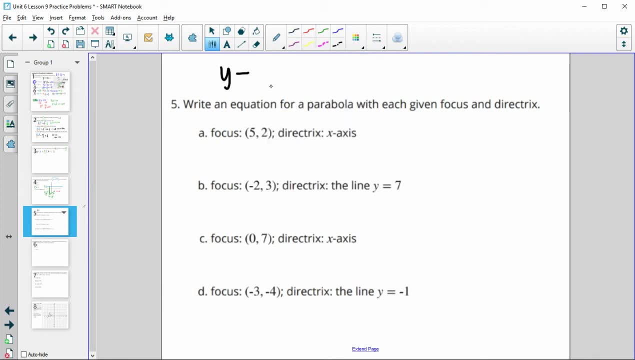 So let's remember how to kind of write this equation. So remember that you do y minus the y-coordinate of the directrix. okay, That gives you the distance to the directrix. Okay, and we square that And that should equal the distance. 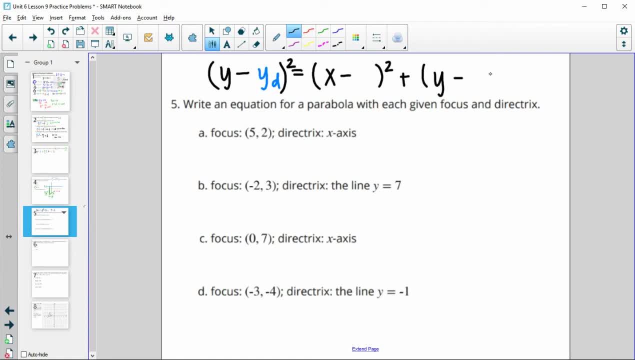 from the focus to the point as well. So we will do x minus the x-coordinate of the focus to give us that horizontal distance, And then y minus the y-coordinate of the focus to give us that vertical distance, And doing the Pythagorean theorem. 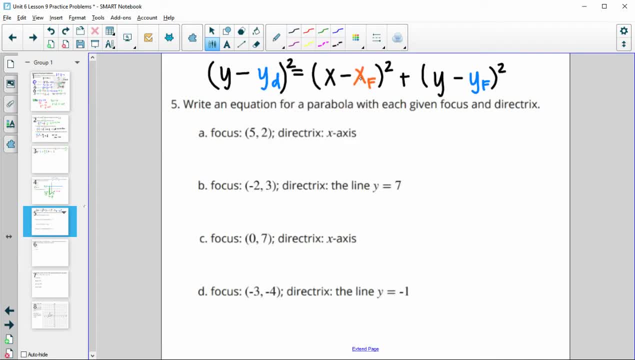 we'll do the Pythagorean theorem here, Okay. so remember that this is giving us that vertical distance. Okay, this is giving us the horizontal, or, sorry, this is giving us the horizontal distance. the orange: This is giving us the vertical distance, okay. 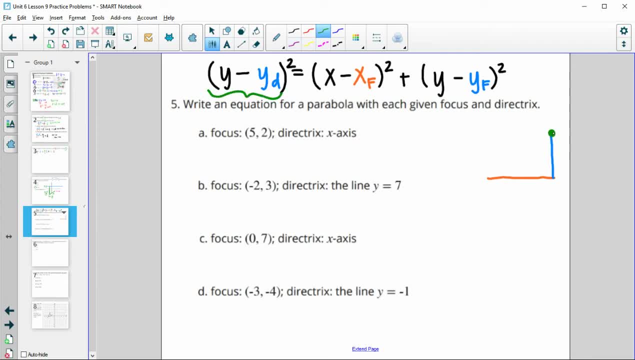 And this right here is giving us the distance to the directrix, and that's the same as the distance to the focus. So, remember, here's your focus, Here's our given distance, Here's our given point. Okay, and this point to the directrix. 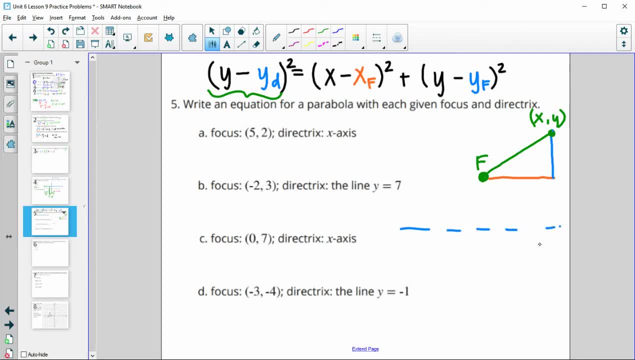 let's just say it's here. We would do y minus this y value. Okay, and that's gonna be the same as this length. So we're doing Pythagorean theorem, So we're just gonna plug into this form here. Okay, so we'll do y minus the y-coordinate. 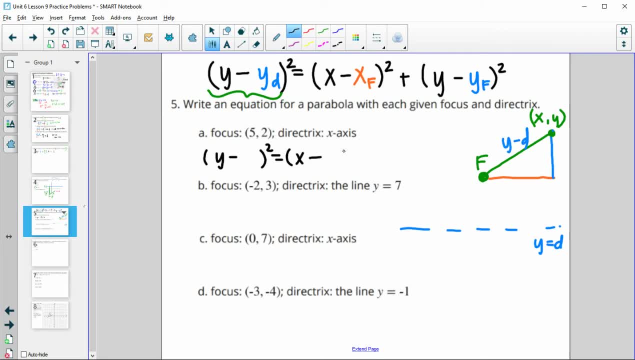 of the directrix squared: x minus the x-coordinate of the focus squared, plus y minus the y-coordinate of the focus squared, So the directrix is the x-axis. That's y equals zero. So y minus zero, x minus the x-coordinate of the focus. 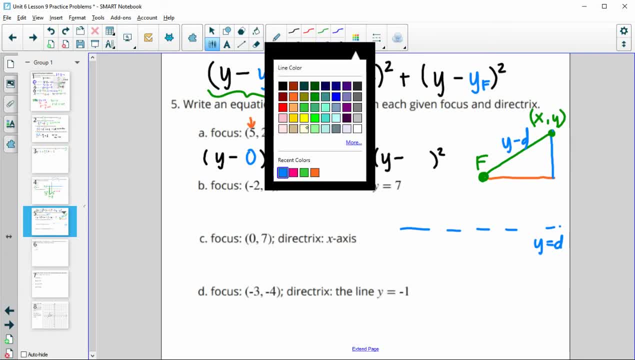 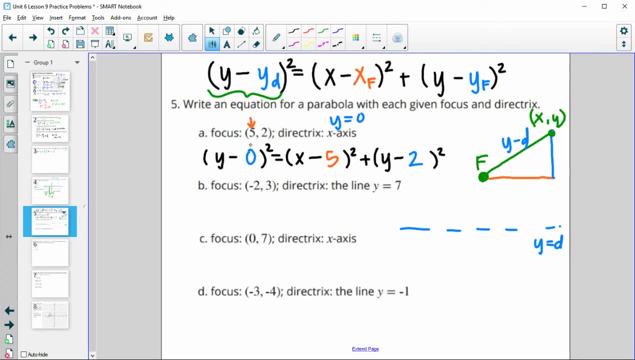 You can certainly change this to y squared, because y minus zero is just y, Or you can leave it And then we'll just repeat this. So y minus the directrix squared equals x minus the x-coordinate of the focus squared, plus y minus the y-coordinate of the focus squared. 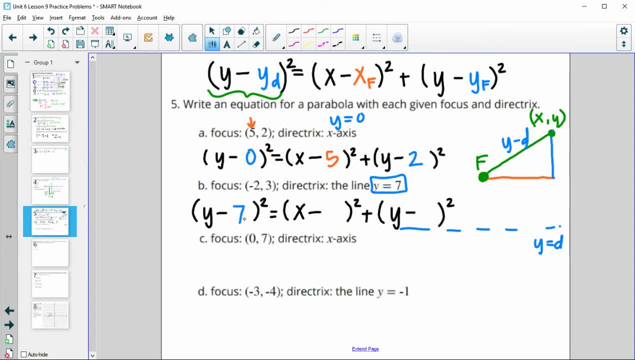 Directrix in this case is seven: X minus the x-coordinate of the focus, So minus negative two, So that'll turn to plus two, And then y minus the y-coordinate of the focus, So y minus three squared Okay. so y minus the y-coordinate of the directrix. 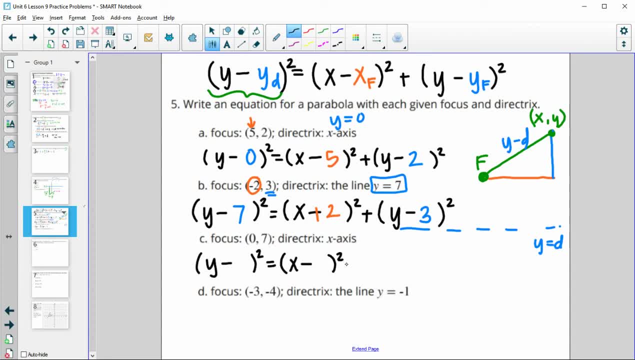 X minus the focus x, Y minus the focus y. So again we have the x-axis. So that's y equals zero. for the directrix The focus x-coordinate is zero. So x minus zero Focus, y-coordinate is seven. So again you can clean these up. 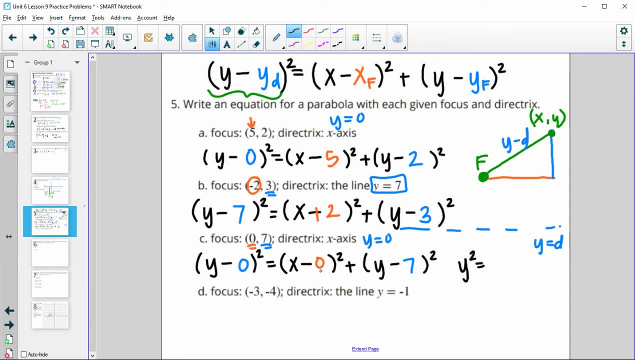 So y minus zero is just y squared, X minus zero is just x squared. And then you have that y minus seven. So you can write it like: y squared equals x squared plus y minus seven squared. if you want to, All right, then y minus the directrix squared again. 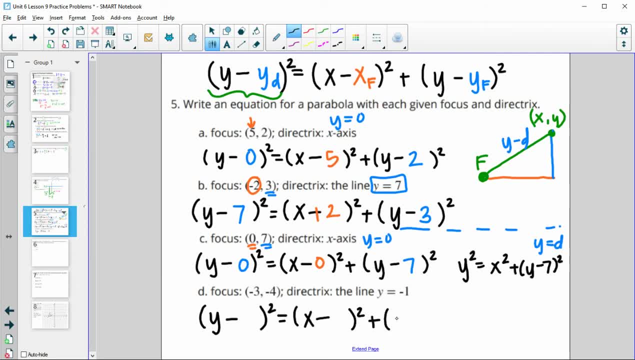 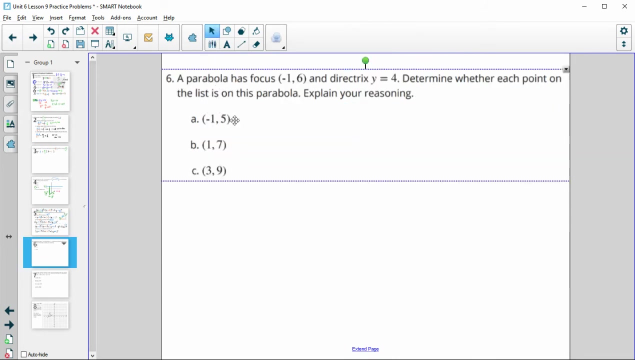 X minus the focus, x, Y minus The focus. y Directrix in this case is negative. one. X-coordinate of the focus is negative. three Y-coordinate of the focus is negative. four. Number six, A parabola, has a focus of negative one. six. 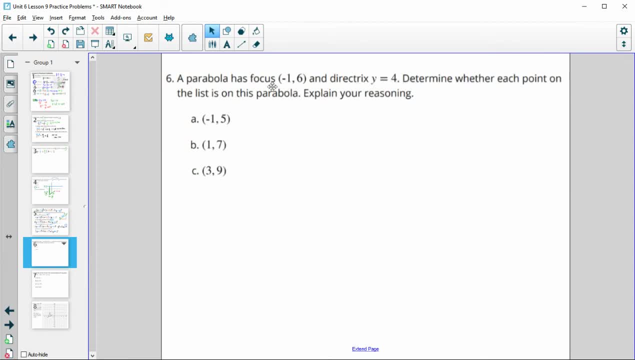 and a directrix of negative one, six. So that's y minus the y-coordinate of the focus, The focus y. The focus y equals four. The focus y equals four. Determine whether each point listed is on the parabola. Explain your reasoning. 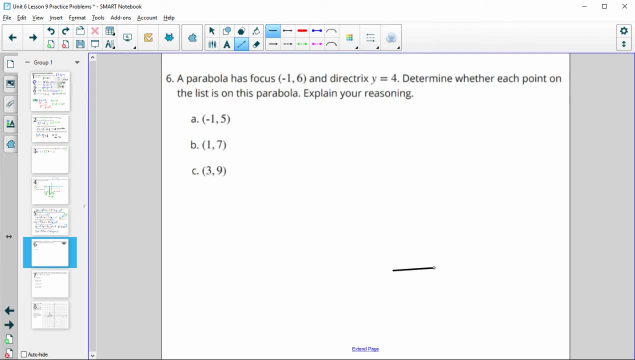 So remember that the focus is a certain distance away from the directrix, And that's where you subtract those y-coordinates. Okay, so here's our focus point at negative one six, And then your directrix line. So is that y equals 4 for this one? 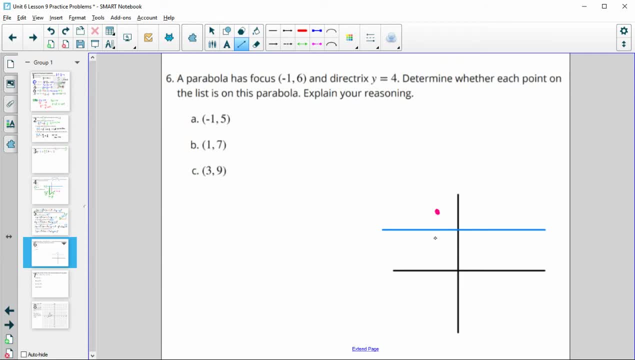 So the focus, the point, is the same distance from the focus as it is from the directrix. And when our directrix is y equals 4,, okay, the distance to this point you're just going to subtract those y's. So the distance from this point to the directrix is 5 minus 4.. 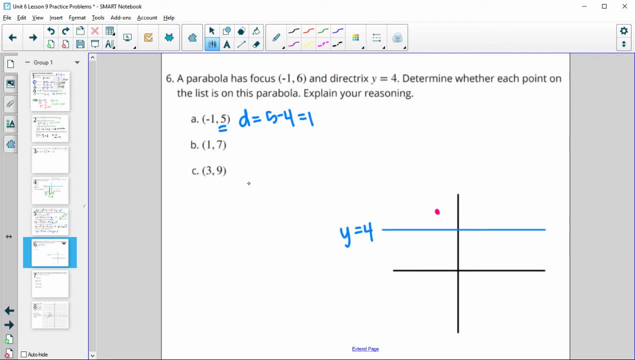 So that's 1.. So then we want to make sure that the distance from this point to the focus is the same. Okay, and this focus point was negative: 1, 6.. So when we go to figure out the distance from this point to this point, we'll subtract the x's. 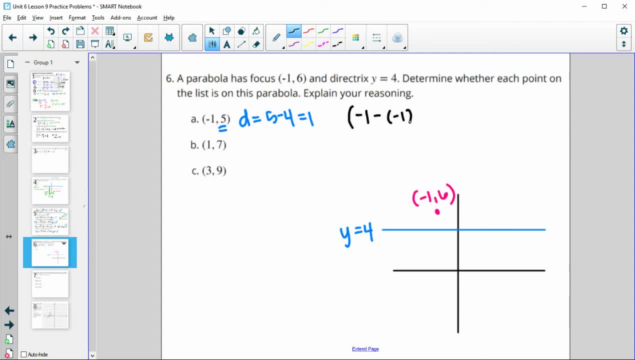 So negative 1.. 1 minus negative 1 squared, And then we'll subtract the y's, So 5 minus 6 squared. That's going to give us this distance, The distance between these two points. So negative 1 minus negative 1 is 0.. 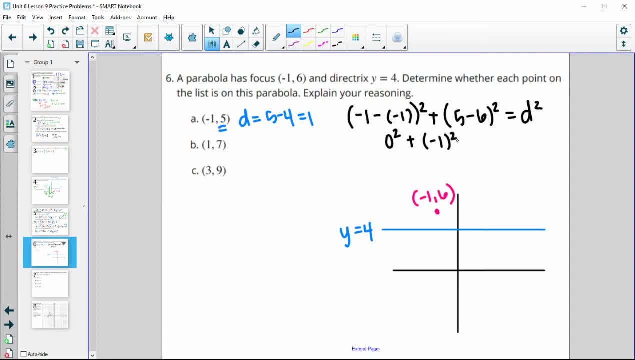 And then we'll square that 5 minus 6 is negative 1 squared. So we get 1 equals the distance squared Square root And we get 1.. So the distance from this focus point to this point is 1.. 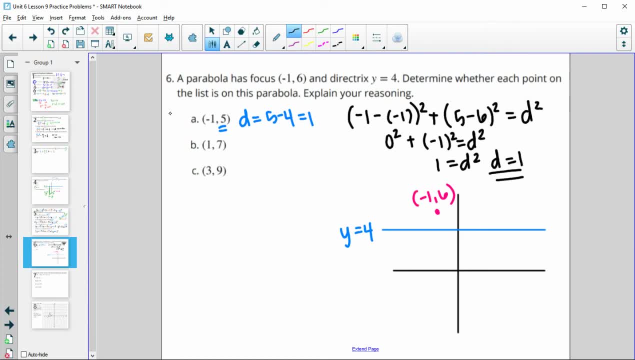 And the distance from the point to the directrix is 1.. So, since those are the same, it is on the parabola, So we'll look at the distance from this point 1, 7.. And you can like plot this: 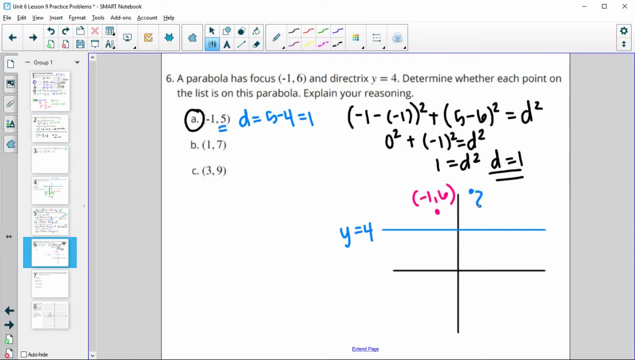 So 1, 7 is here. So you're trying to figure out this distance. So we're taking 7 minus 4 to figure out that distance, which is 3.. Then we're trying to come up with the distance between this point and the focus. 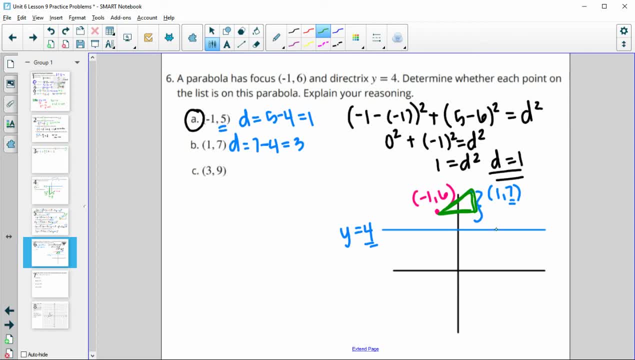 So we're drawing in this little right triangle, Okay, figuring out the width here by subtracting the x's, So negative, 1 minus 1 squared, plus subtract the y's, 7 minus 6 squared, So that's going to be, and you can call it distance squared, okay, or you can call it the c value, but we're finding that hypotenuse. 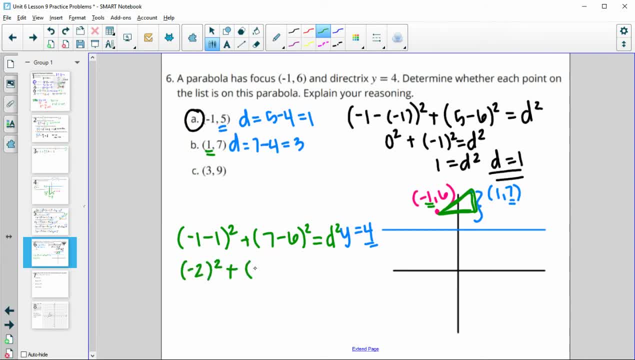 So here we have negative 2 squared. 7 minus 6 is 1 squared, So we have 4 plus 1 equals our distance squared, So 5 equals d squared. So the distance between these points is the square root of 5.. 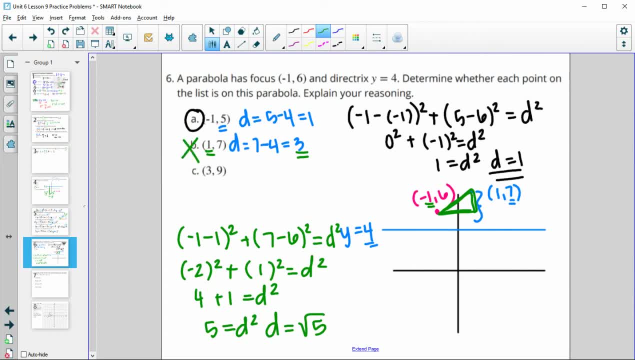 That is not the same as 3,, so this is not on our parabola. So then this final one, again the point 3, 9,. okay, so if we're at 3,, 9, and we can't really see this with all the rest of this, 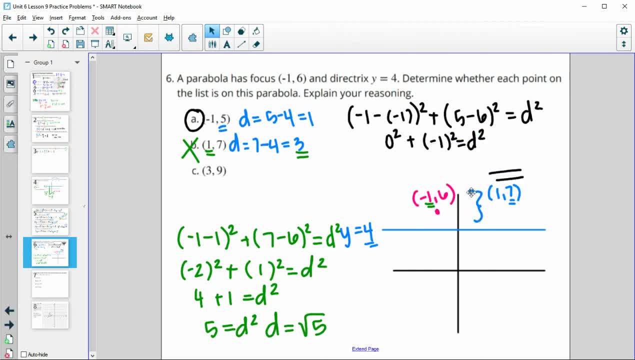 Here's. let me delete some. So if we plot this new point, 3, 9, okay, so 3, 9 is going to be here. The distance from 3, 9 to this directrix at y equals 4, we'll just subtract those y values. 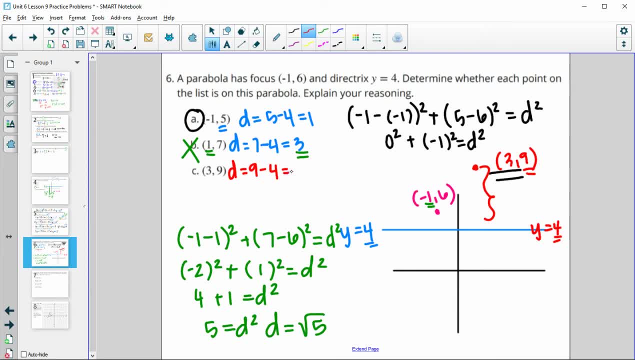 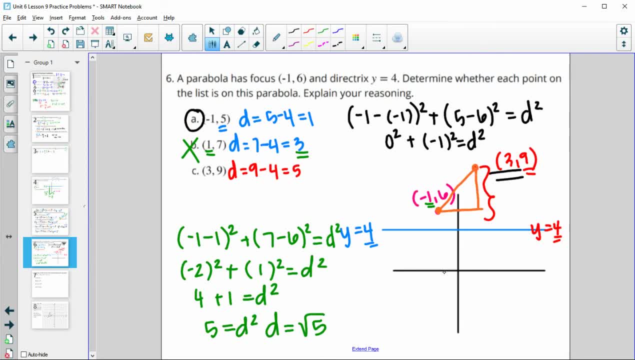 So again we'll look for the horizontal and the vertical distances by subtracting the x's. So we'll subtract these x's negative 1 minus 3 squared, And then we'll subtract the y's 6 minus 9 squared. 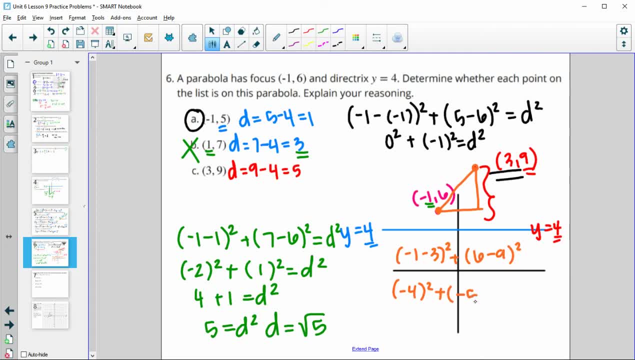 So we have negative 4 squared plus negative 5.. squared will be this: distance squared So 16 plus 20.. Oops, Sorry, I have this wrong. I spoke wrong. This is three, So this is negative three squared. So nine, 16 plus nine is 25, is our distance. 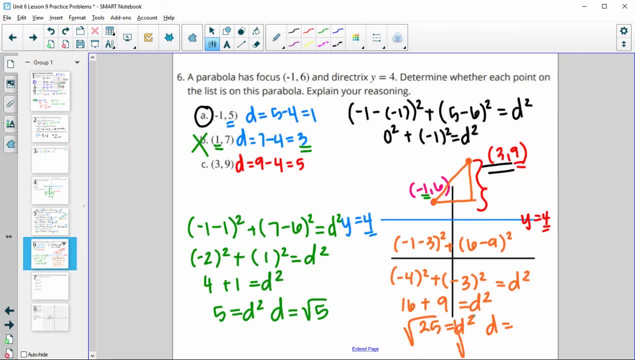 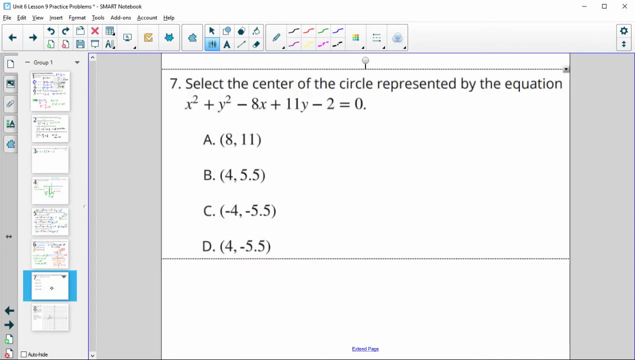 squared. So then we'll square root that And we'll get our distance equals five, which is the same as the distance from the point to the directrix. So this one is on our parabola. Number seven: select the center of the circle represented by this equation. So we're going. 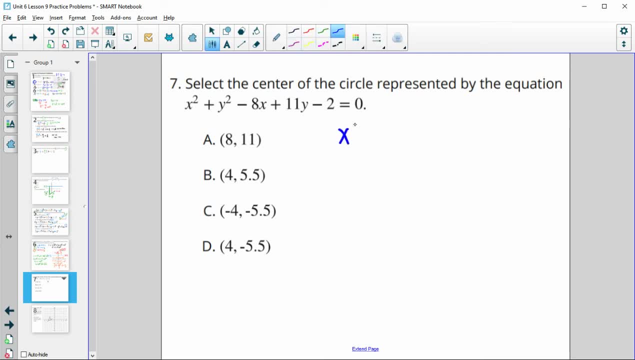 to want to look at completing The square. So we'll put the X's next to each other and leave a space for that C value Whoops. And then I'll put the Y's next to each other, So we have Y squared plus 11 Y. 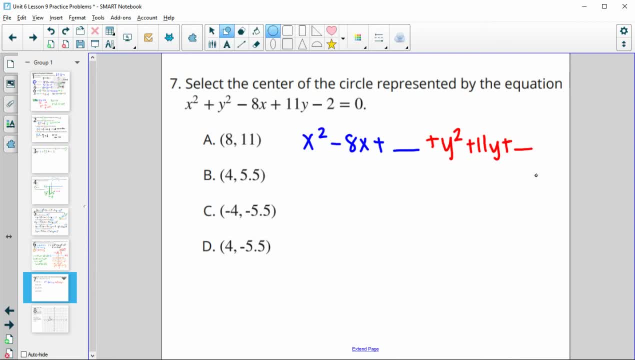 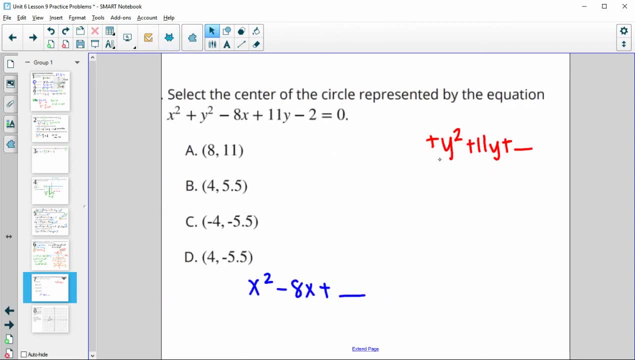 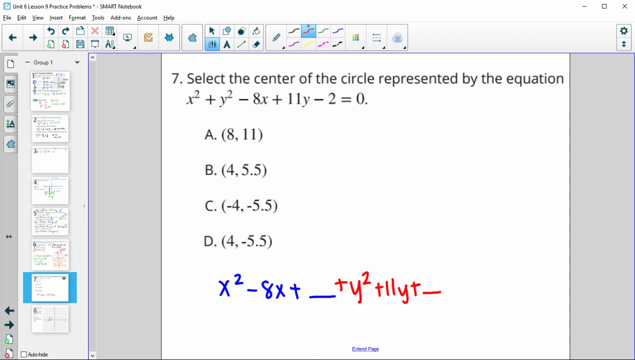 And then we would have another term here. Actually, why do I keep grabbing the circle? Um, I'm going to move This down here So I can have some more space. Um, and then I would add this two to the other side. 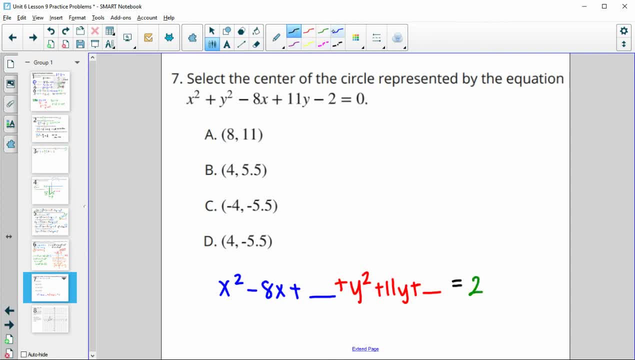 So we'd be at two, And then we'd have um blanks for each of these For when we're going to complete the square. Now we don't actually need to find the radius here, So we don't have to do the full process. 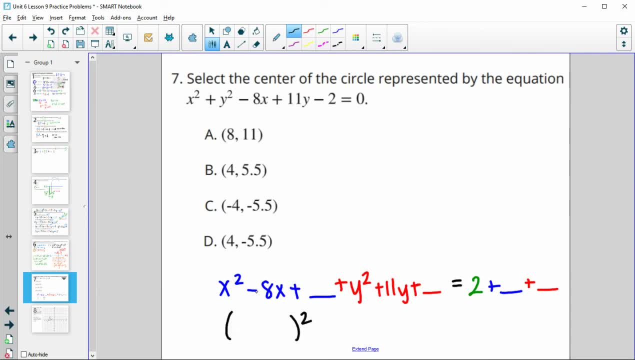 Okay, If you think about what would this be when we factor it, when we factor this down, This is going to be X minus four squared, So this would be a 16 if we want to complete the whole process. And then for this one, we'd have 11 divided by two. 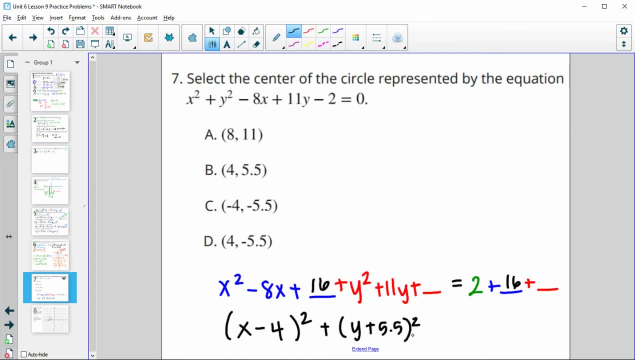 So we'd have 5.5 squared in here. So now we actually already know the center without having to finalize the radius. So if you don't want to finish the whole process, your center is going to be four. Okay, so positive four. so not this one or this one, And your y coordinate is going. 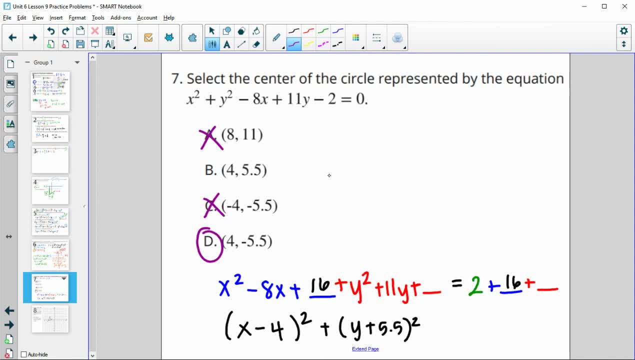 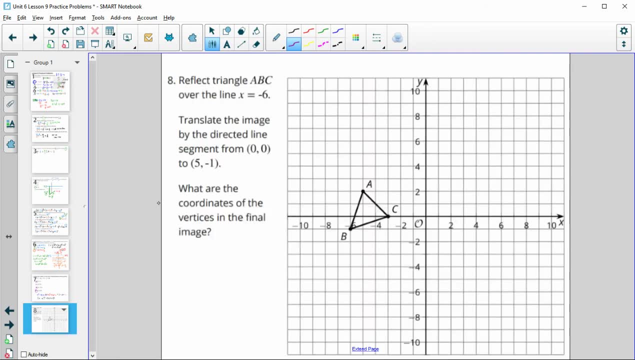 to be negative 5.5.. So this is going to be your center, without actually having to complete the whole process. All right, then. number eight has us reflect over the line. x equals negative six. So here's: x equals negative six. So we're just going to reflect these points over that line. 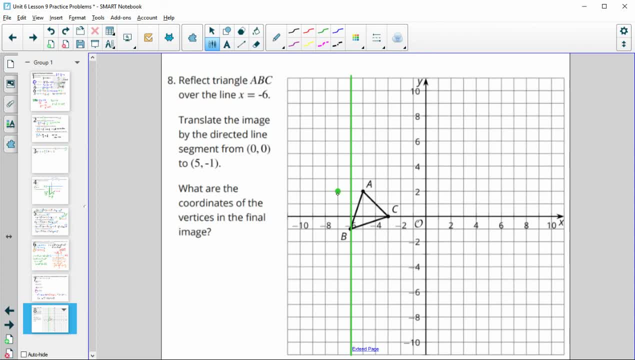 So a is one to the right of the line, So a prime is going to be one to the left. b is on the line, So b prime is going to be on the line. c is three to the right, So c prime is going to be three to the left.